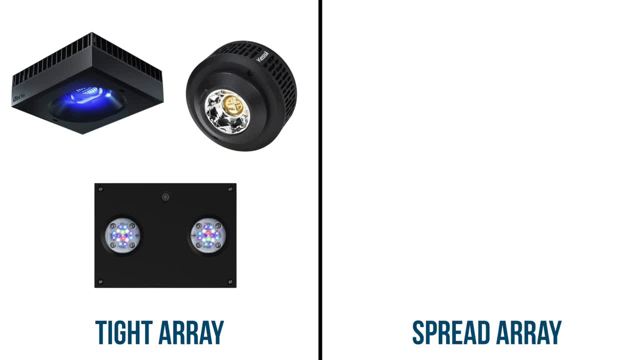 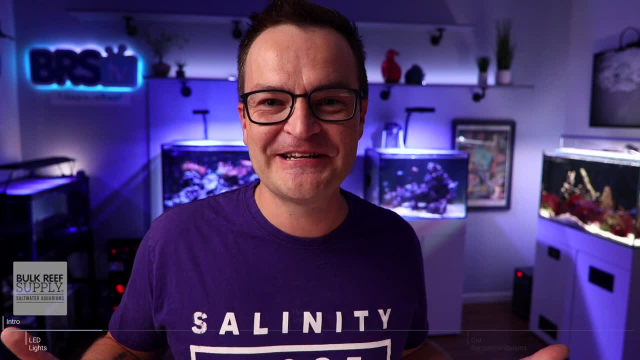 of their LEDs in a small area, Or should you go with an LED panel that has the lights spread out over a larger area, such as the Reef Breeders, the Reef Brights or the Orfec fixture? I mean seriously, how is a beginner supposed to navigate this world? You might have one fixture. 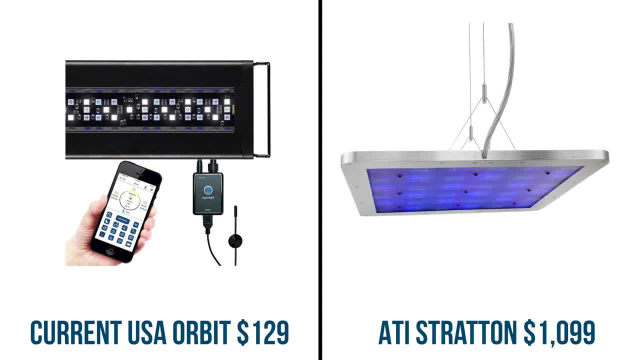 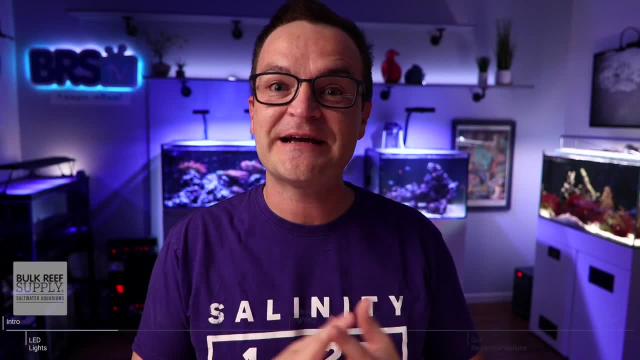 that looks good for $100 and another fixture that looks good for $1,000.. And, as a beginner, you're just going to have no idea And you're going to want to rip your hair out and walk away from this hobby because it's so confusing. So I'm going to try to make this as simple as 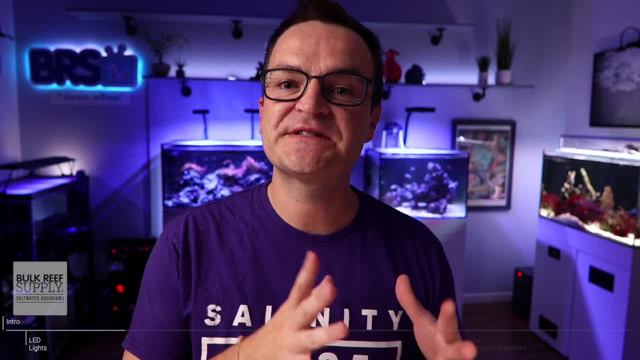 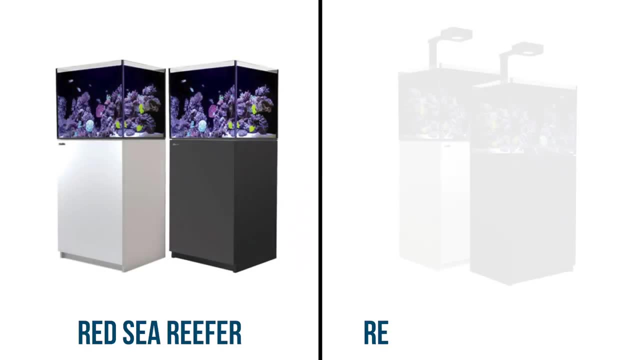 possible for you. The first thing I'm going to recommend is, if you buy some sort of all-in-one system- let's say you buy a Red Sea system or any other system that has an option to purchase lights with it- buy those lights, because then you will know that. 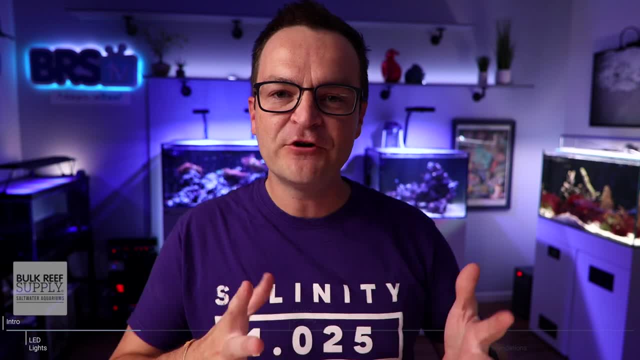 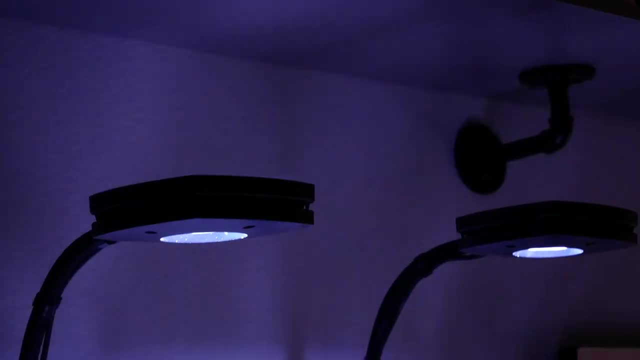 the lights will definitely work for the size of your tank. If you're building your own system, I would honestly recommend just sticking with the Aqua Illumination lights. They are a middle of the road light, They're not priced too high and they've been shown to grow a whole bunch of. 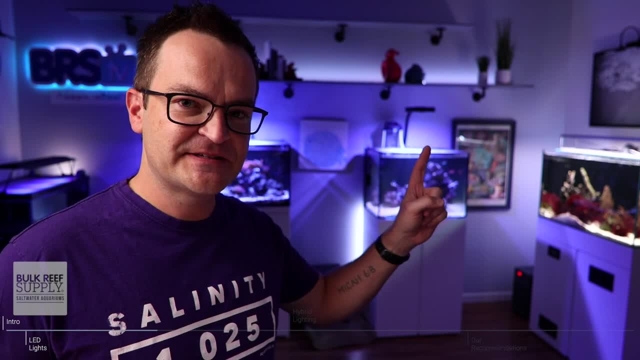 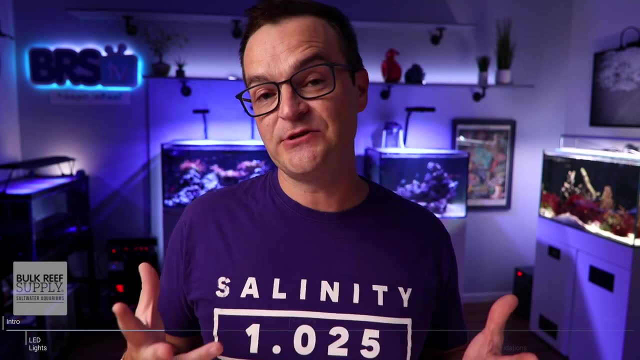 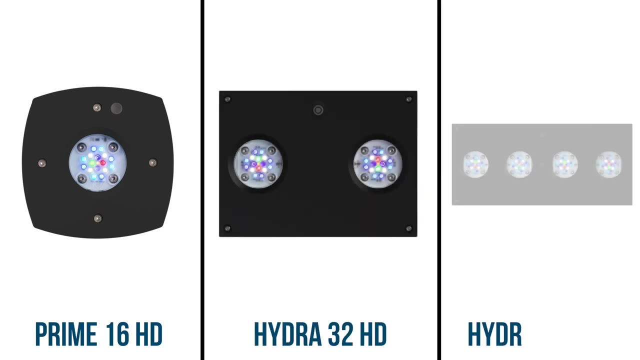 corals. If you're curious what they look like, this is a Hydra 32 by Aqua Illumination and these are 16s by Aqua Illumination. I use them myself and I really like them. They come in different sizes, from the Hydra 16 all the way up to the 64. And really all you need to do is purchase the correct. 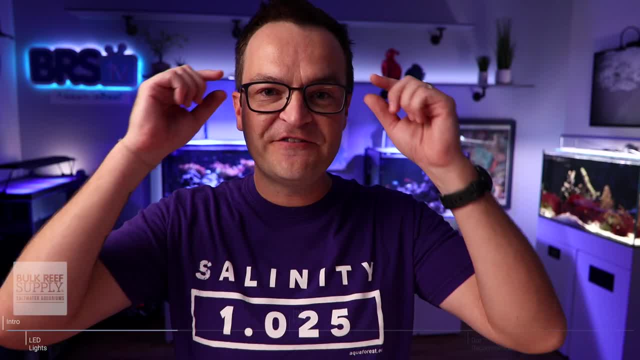 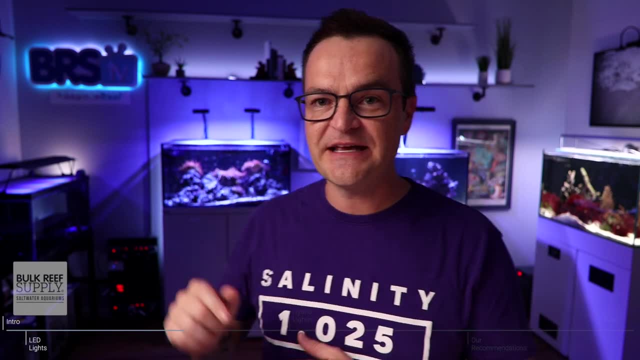 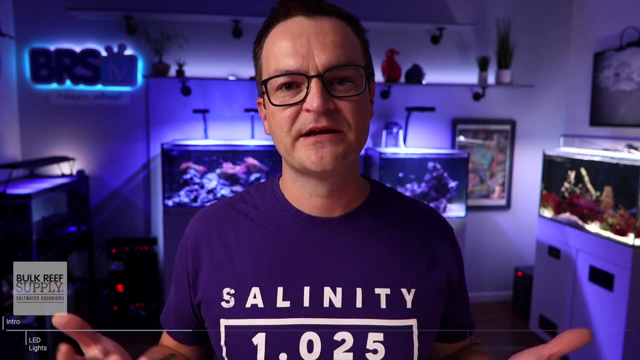 size and the correct number for your tank. So the most difficult decision you're going to have to make is: if you have a slightly larger tank, do you go with two of the 16s Or maybe, instead of that, do you go with 132 or 164?? And if you have any questions, all of us here at BRS are here to 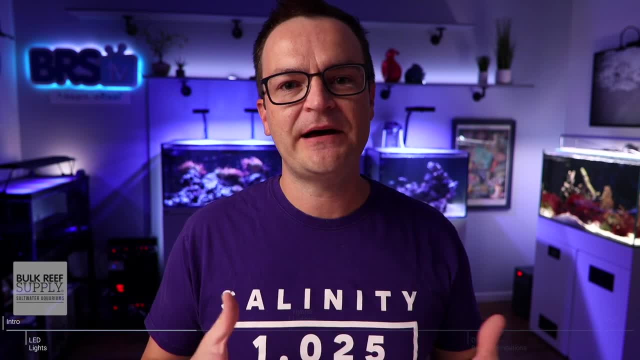 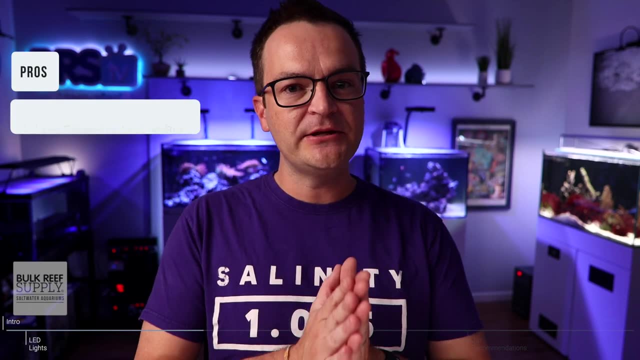 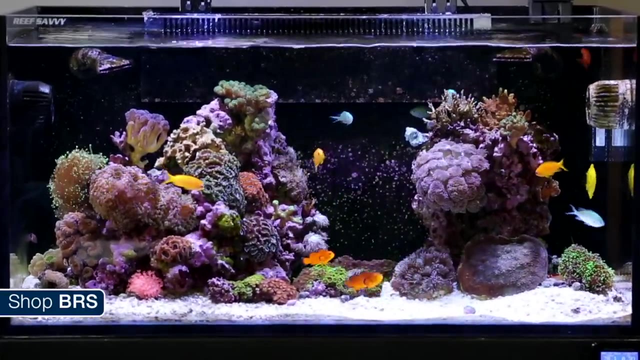 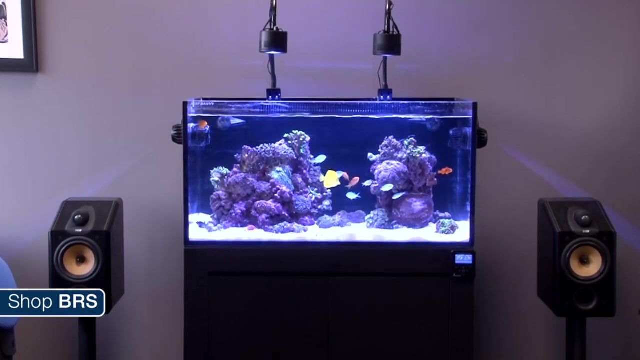 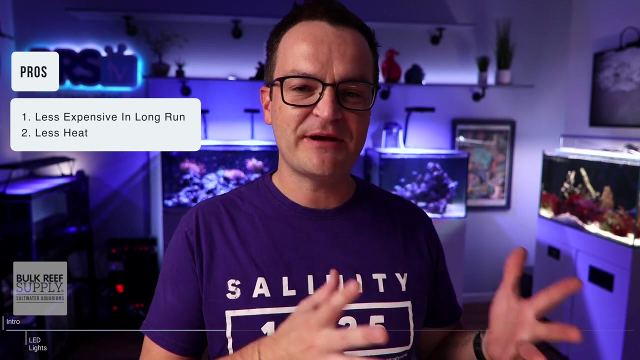 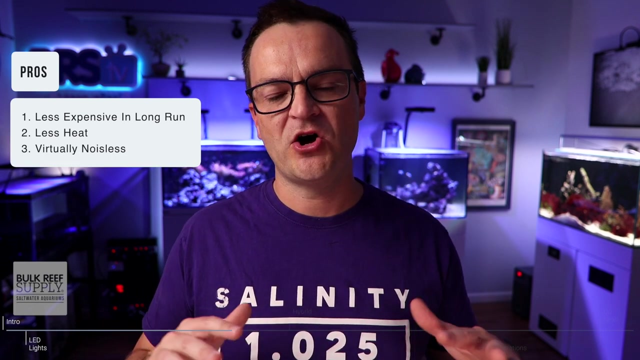 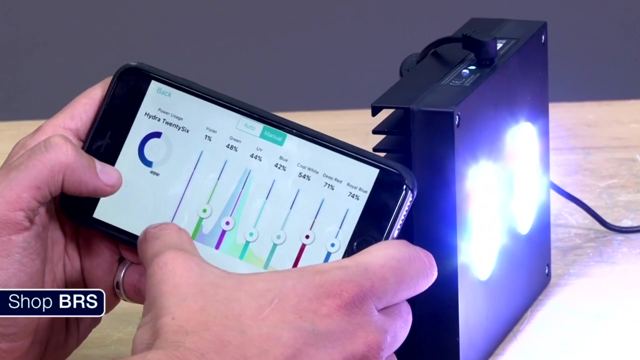 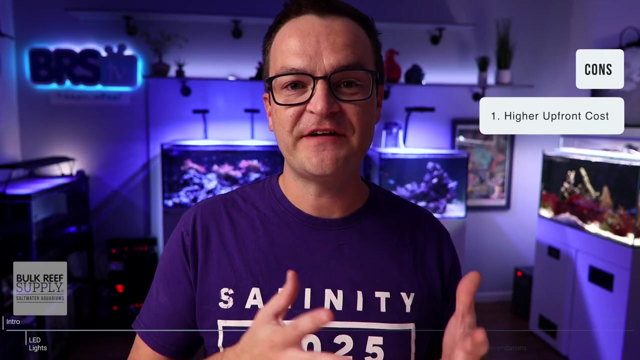 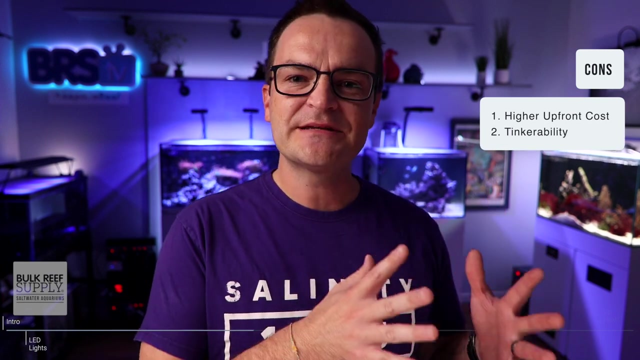 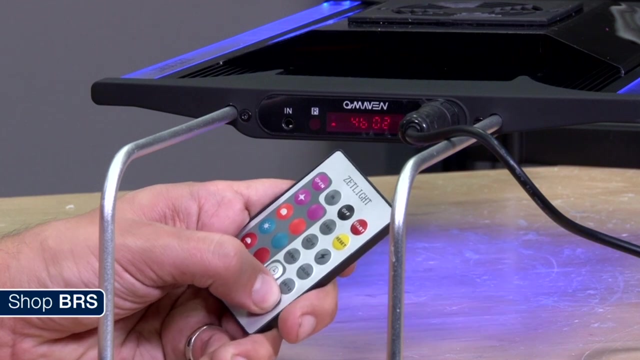 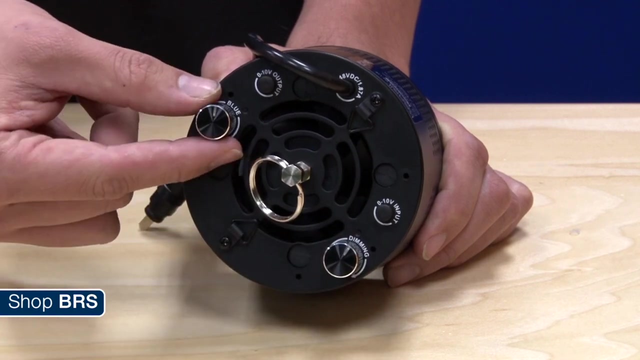 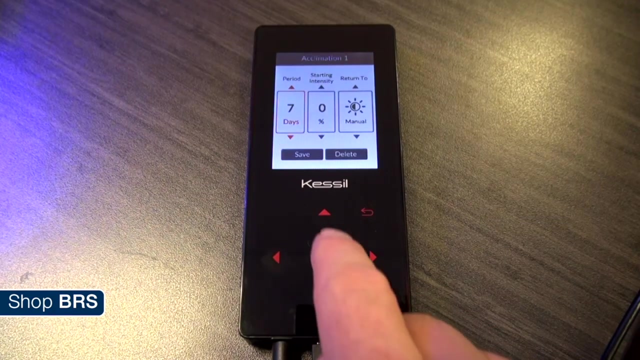 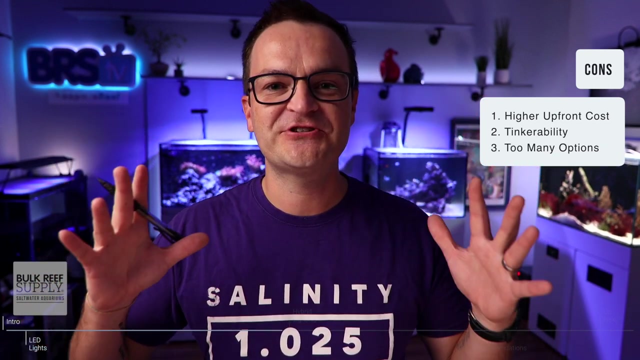 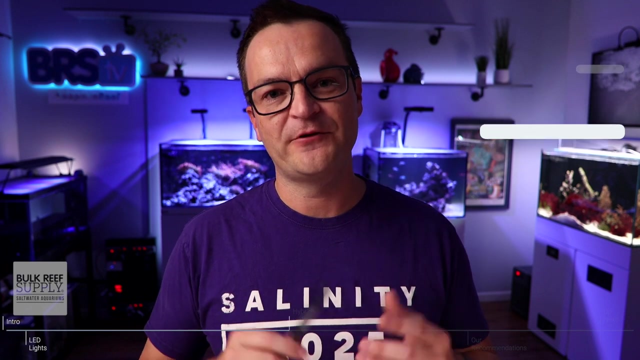 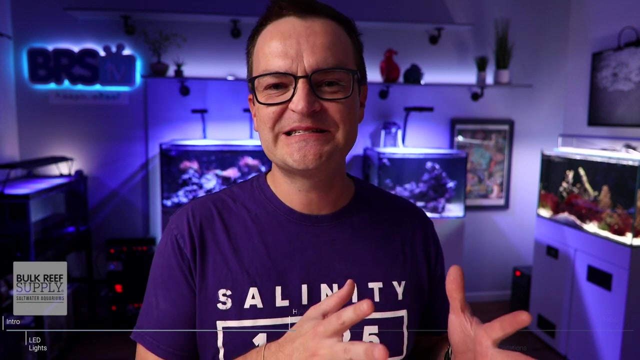 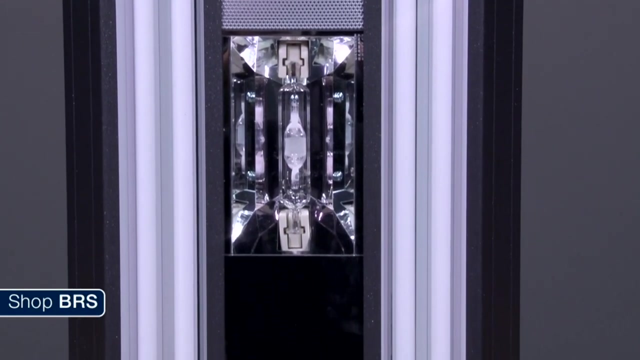 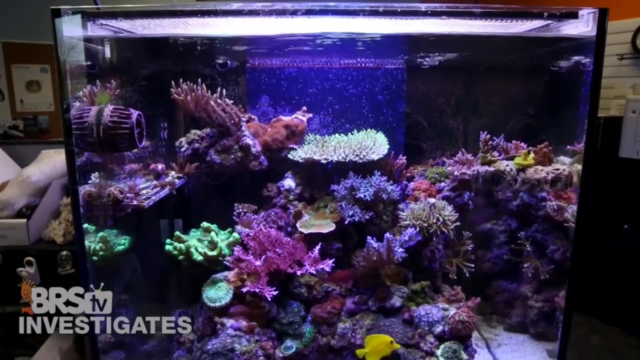 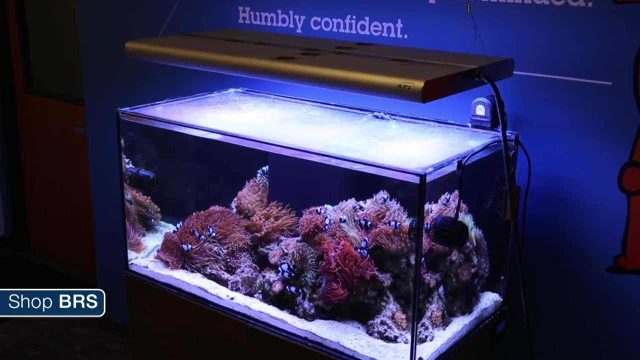 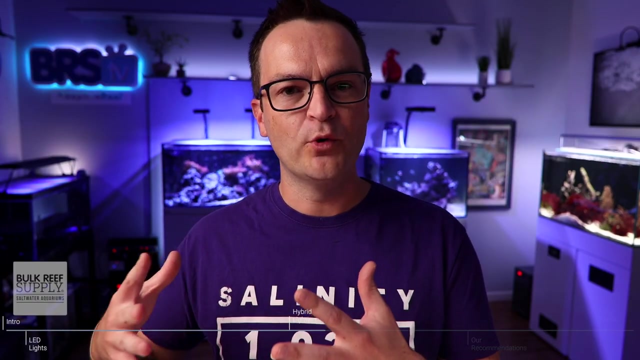 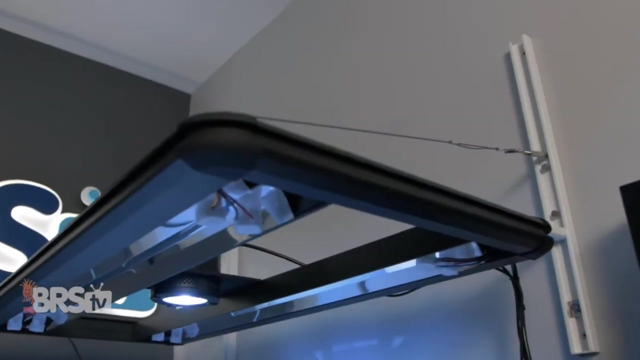 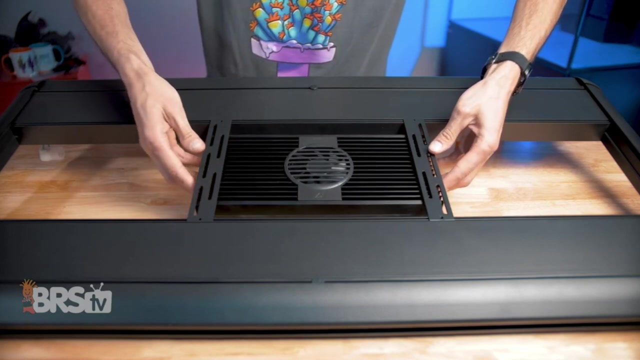 help you out. If you have any questions, feel free to reach out to me at BRScom And I'll see you in the next video. Bye-bye, Bye-bye, Bye-bye, Bye-bye, Bye-bye. 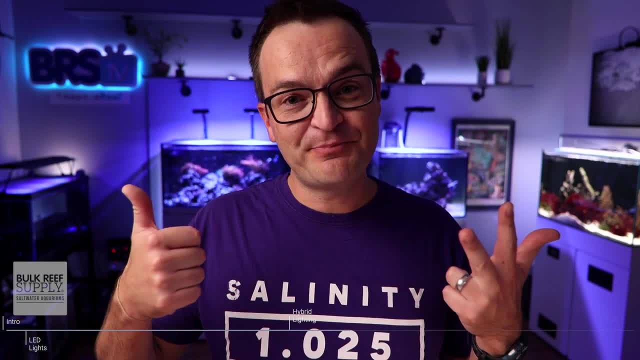 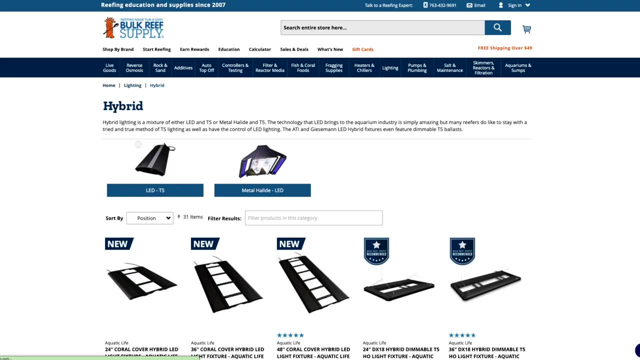 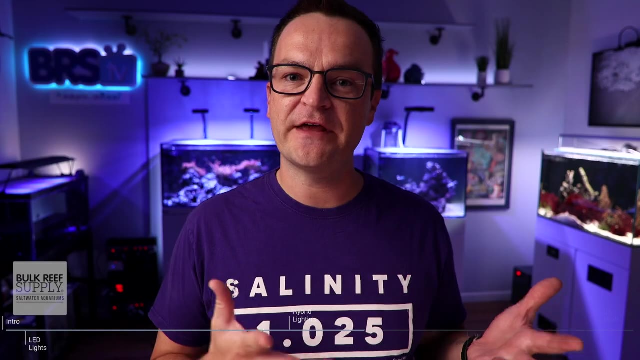 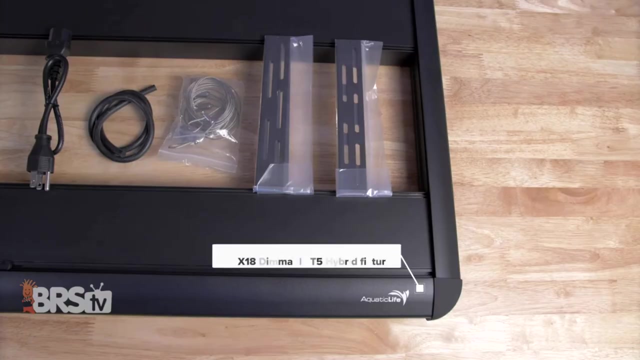 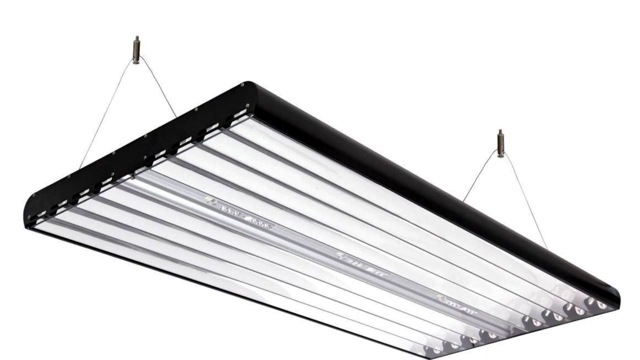 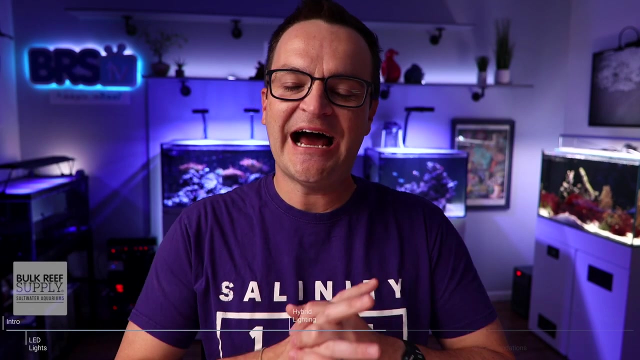 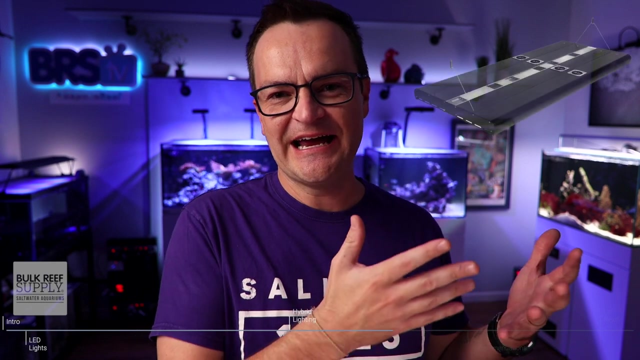 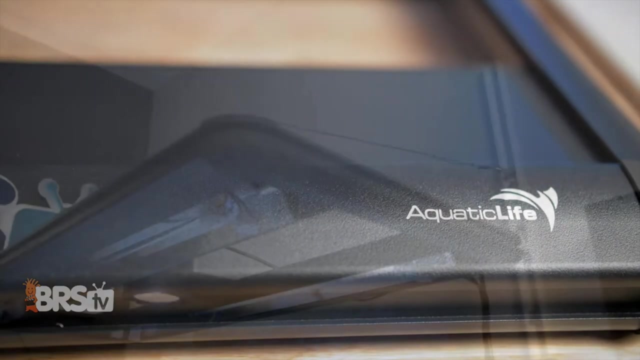 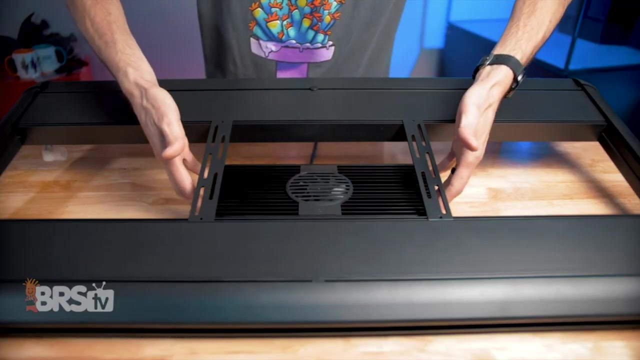 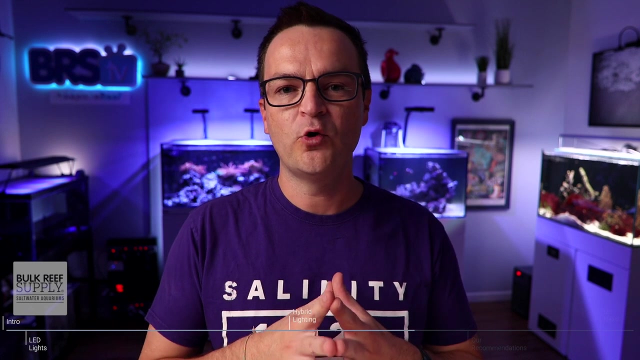 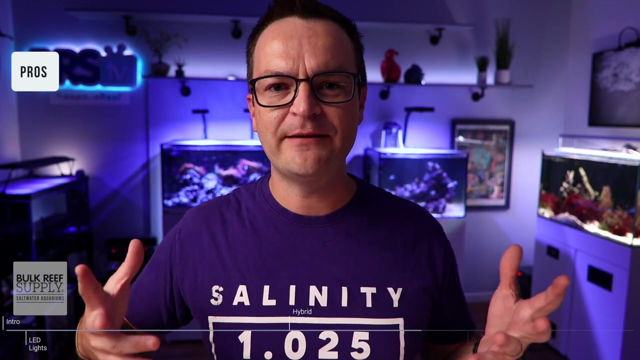 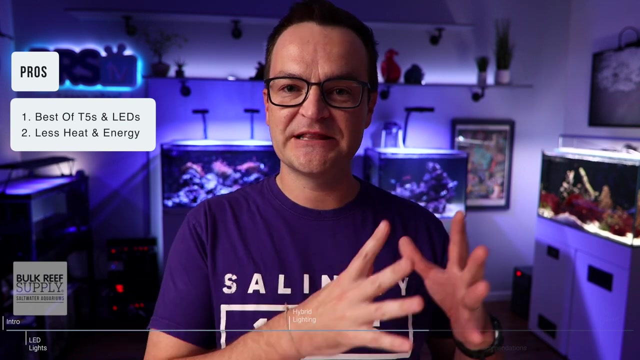 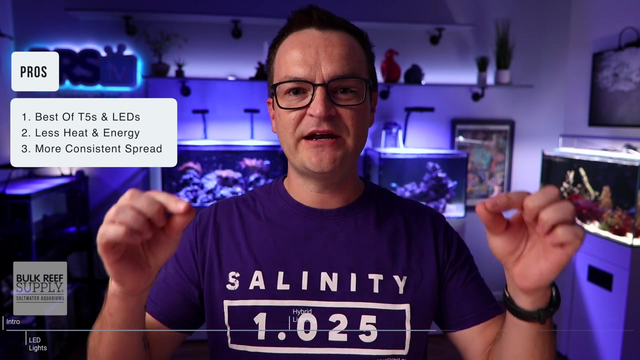 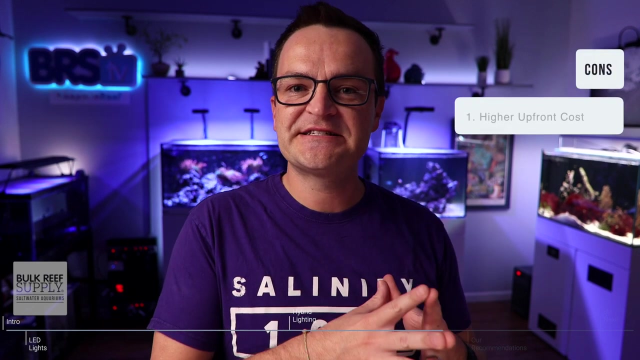 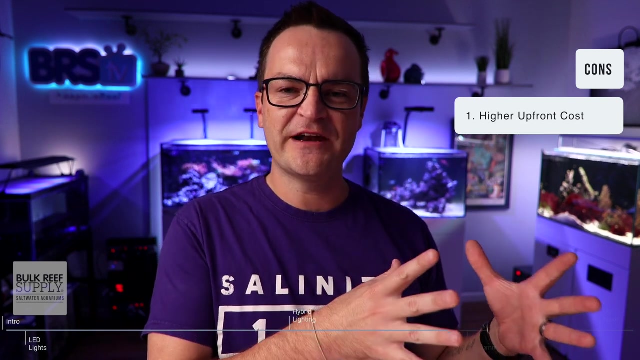 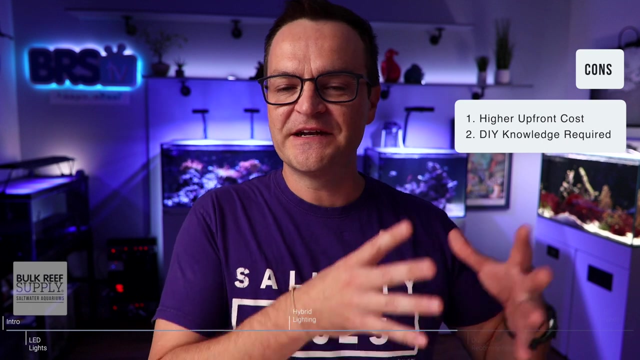 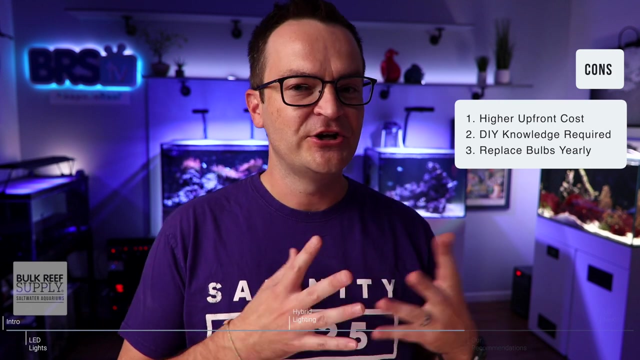 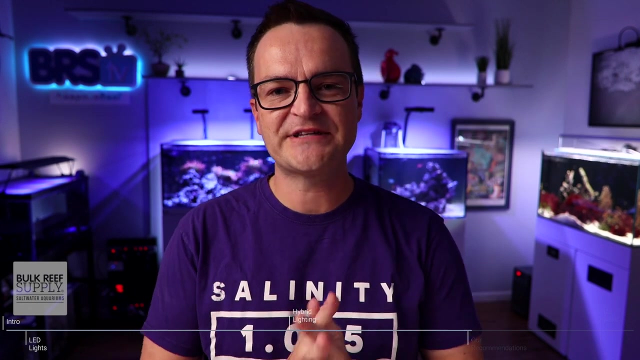 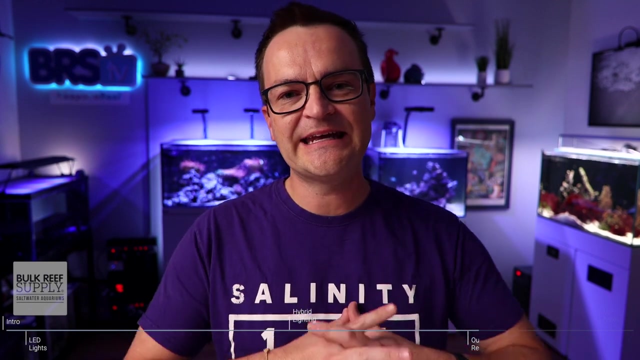 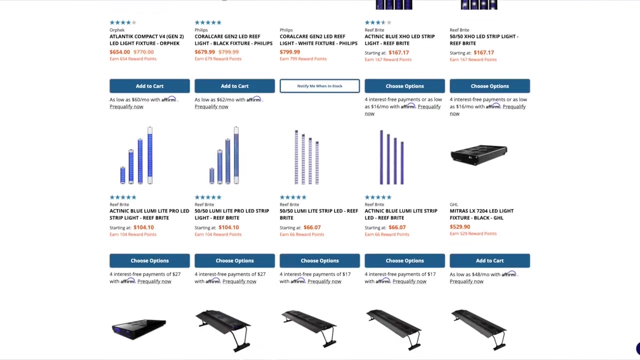 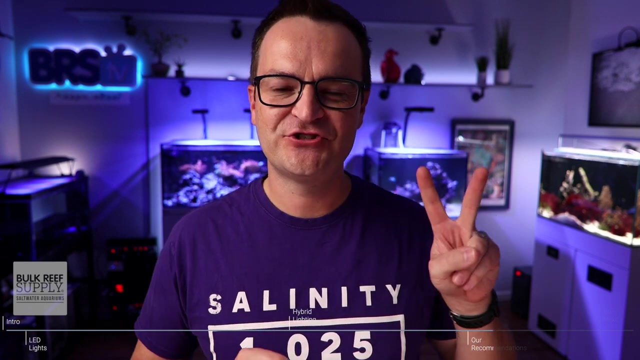 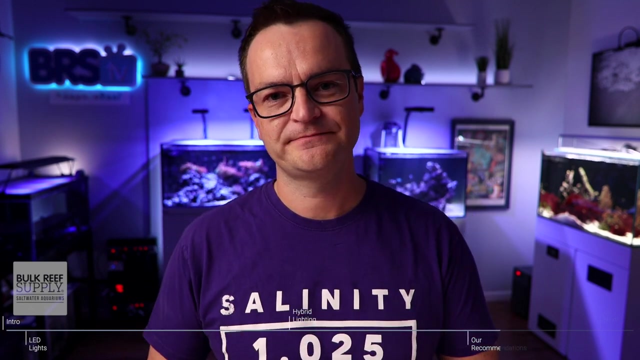 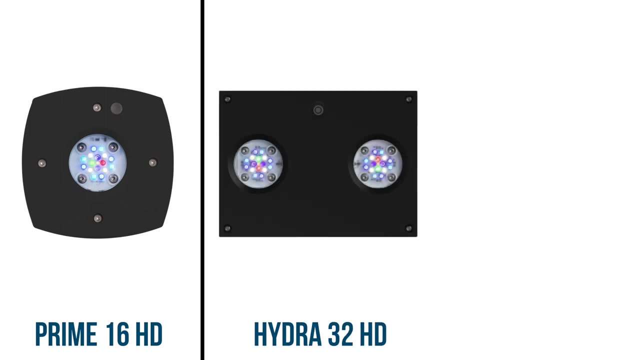 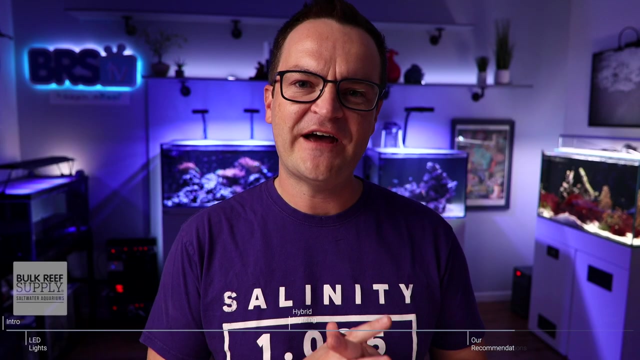 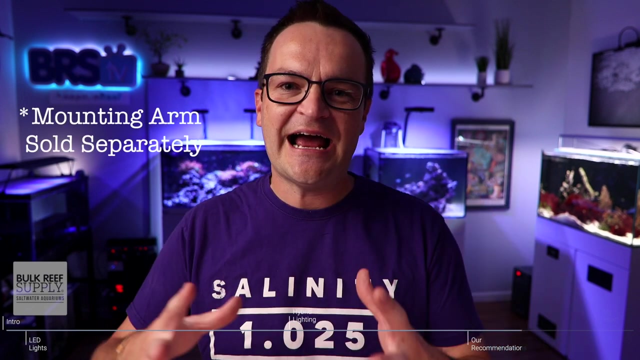 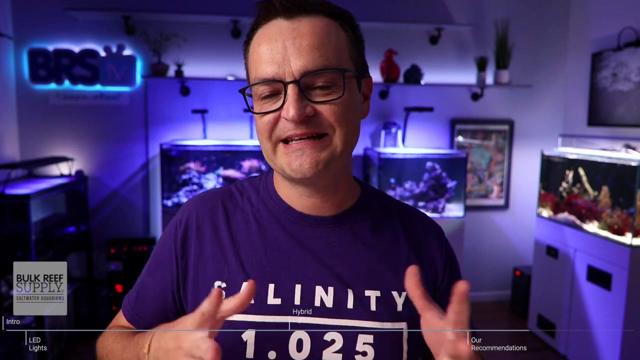 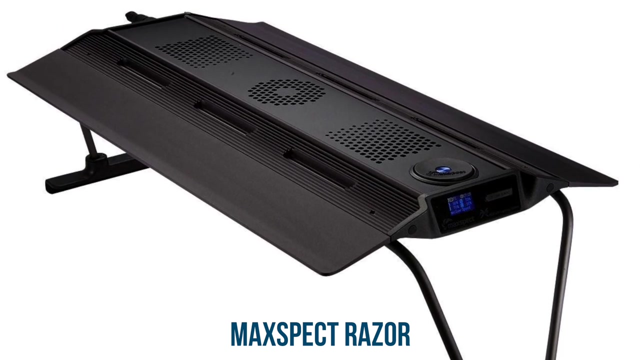 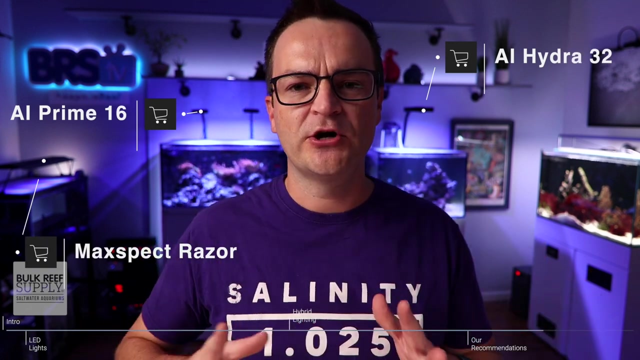 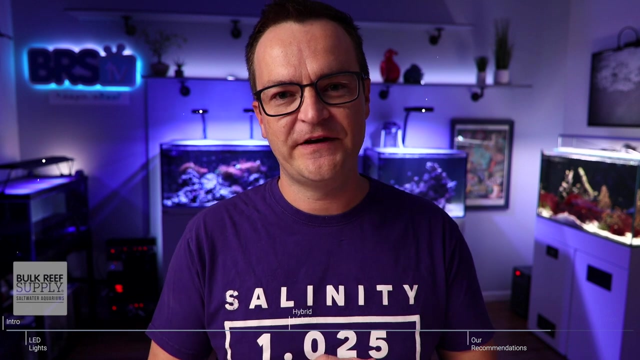 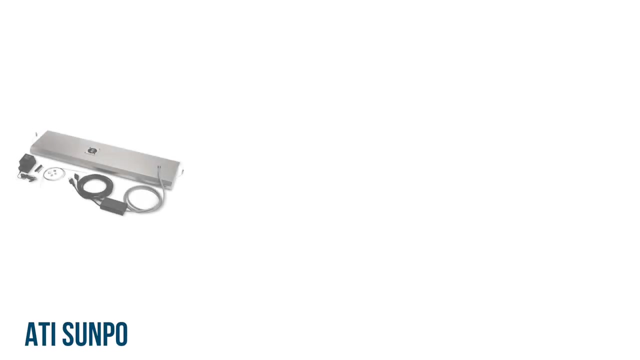 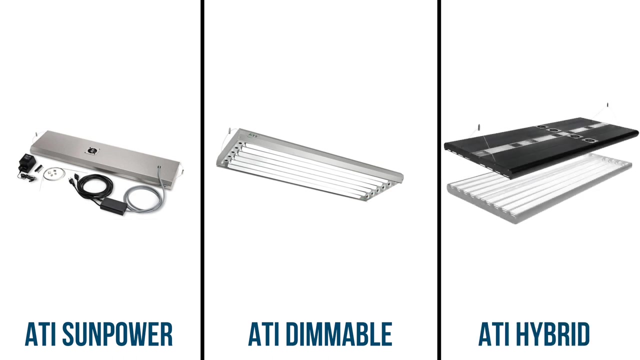